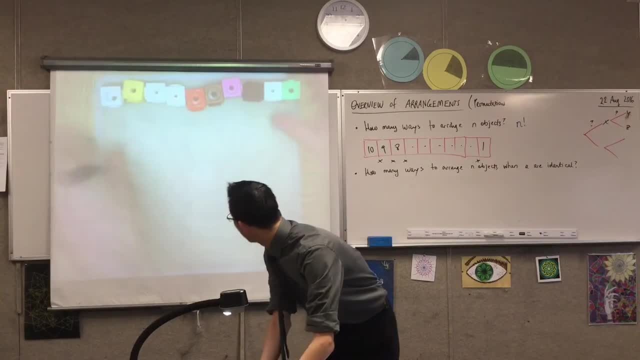 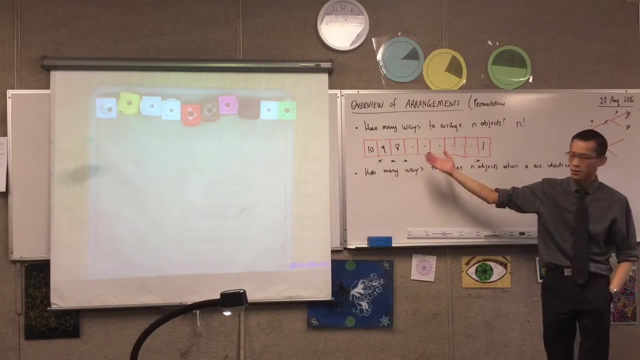 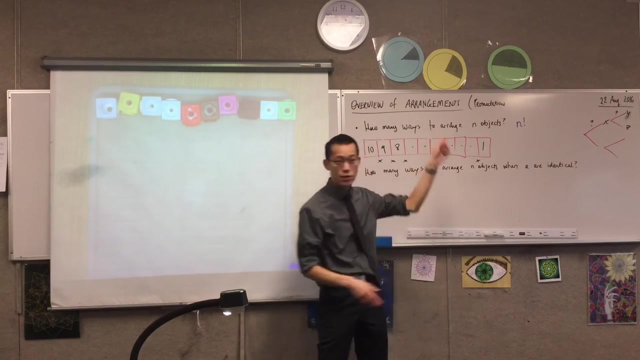 And eventually they fit. There we go, Eventually I get an order Okay. So I'm like, look, there are 10 factorial ways that I could do something like this, But then you notice. then you notice When you have a look, because the most important thing that differs from here to the previous one is clearly these guys right. 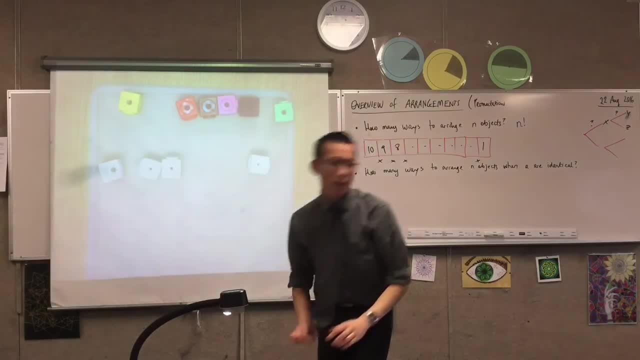 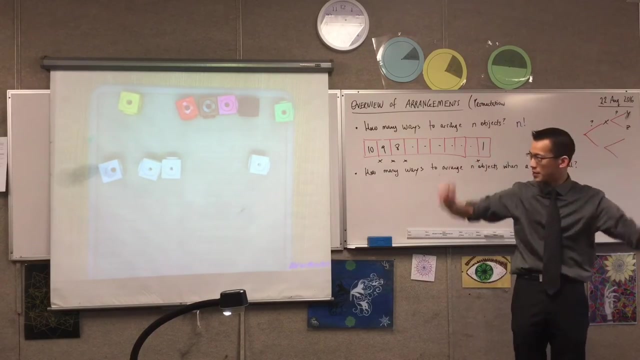 These guys here. Let's just break them out for a second. Okay, Now these identical objects you can see Like as an arrangement, right, These guys are kind of their own arrangement. This is an important idea in arrangements that you've got like sub-arrangements within a big set of arrangements. 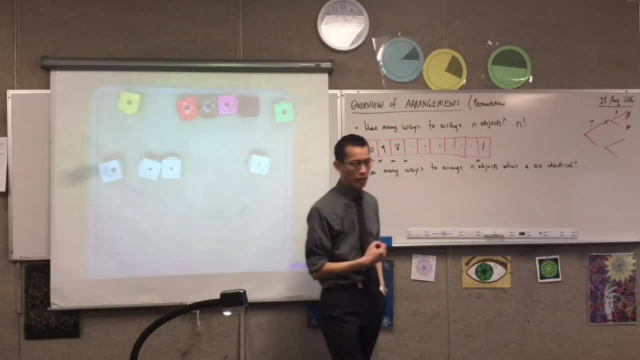 And you can see these four I can also put in a particular order. Do you notice that? Now hold on a second. Go back to this one. How many ways can I arrange these four identical objects, Four factorial right? 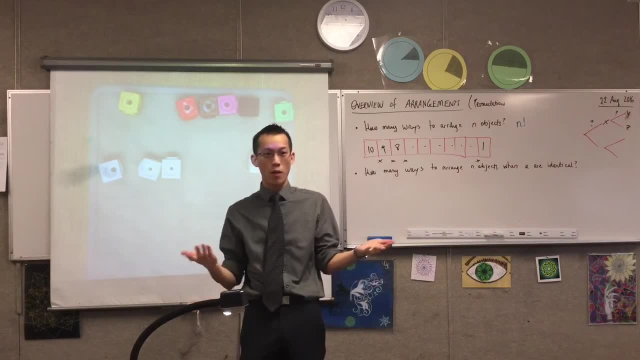 Four factorial. But as soon as I do that, for example, think about: oh, what's a different way. I could do it Like say, maybe I swap these guys and then I swap these guys, So I've got a new arrangement. 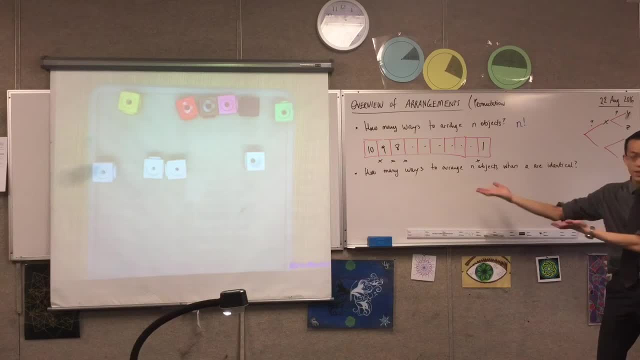 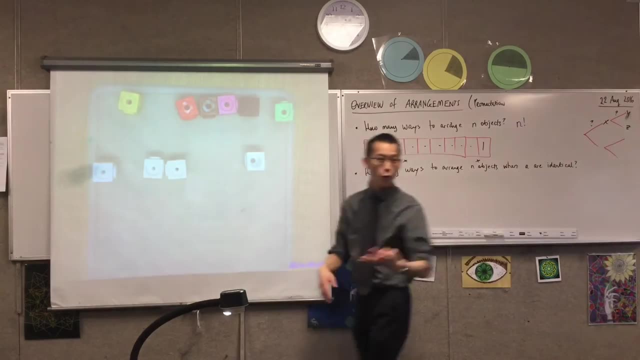 Except for the fact that this is exactly the same as well, to my eyes, right, This is exactly the same as the arrangement I had before, And I can do this, I can rearrange these guys four factorial ways. So, therefore, I'm not going to get good morning, I'm not going to get ten factorial. 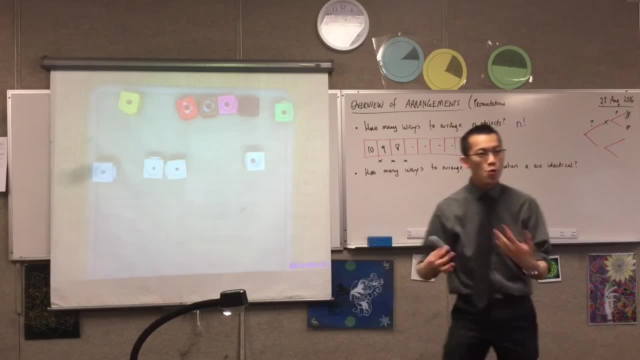 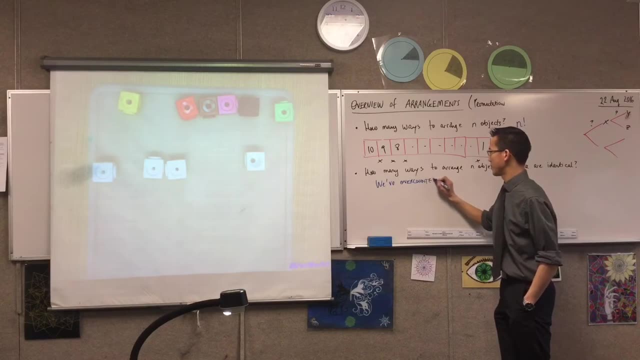 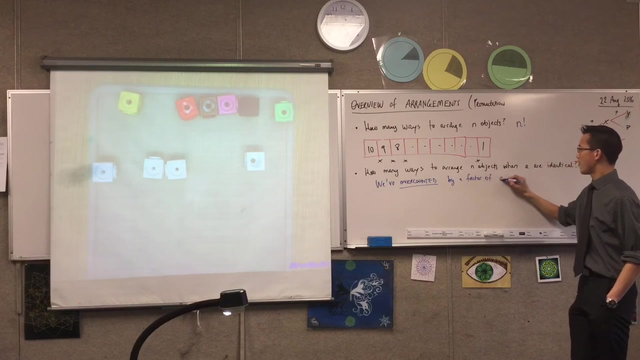 I've actually- and this is an important idea- I have overcounted right, We've overcounted. This is such an important thing. No, no, no, Capitalize it, Underline it. We've overcounted by a factor of a factorial. 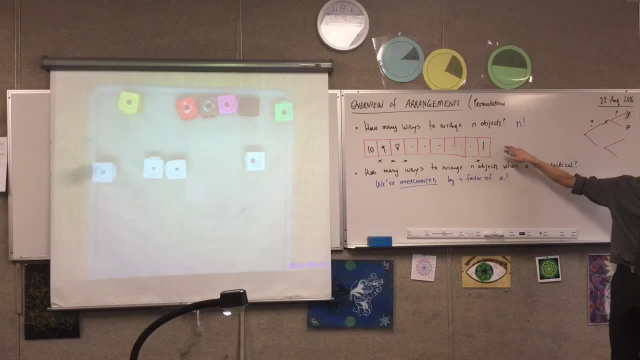 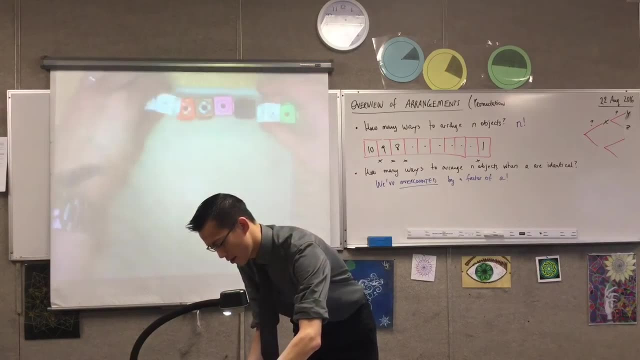 Okay, So this is different to when I had a look here and I was like, well, how many spots have I got? I still had to fill up all the spots. I still had the same number of objects, Right, Yeah. 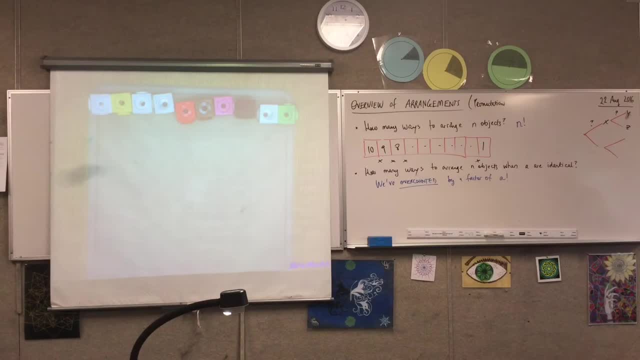 I want to ask: what about if the a factorial minus one? because, like, if you take away four factorial from that, I mean like there would be you know more, as if it would be back. What do you mean by blanks? 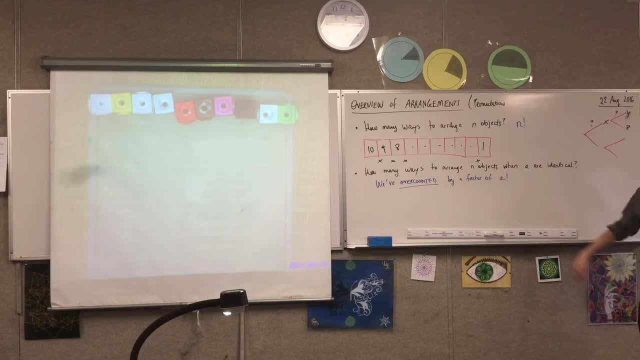 I mean like, if you like, by thinking out like four factorial, that means that you don't have a blank. Do you know what I mean? Okay, so the idea is that I suppose part of the problem is the language we're using here, right? 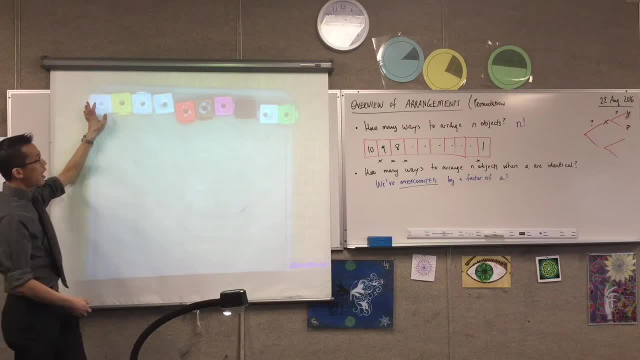 When I said: oh, I take out four factorial, I'm dividing by four factorial right. So what I'm thinking about is all the different ways I can have this exact same one here and the white ones are still there. It's just like: well, the white ones can be rearranged in four factorial ways. 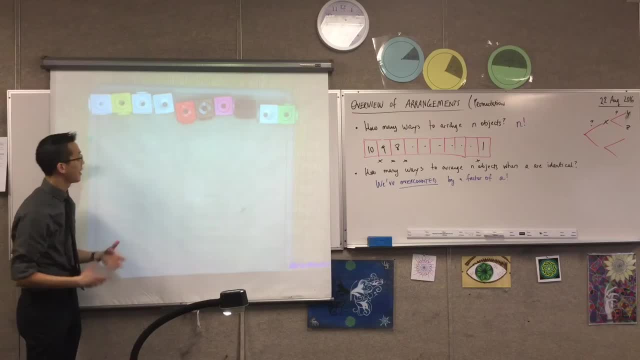 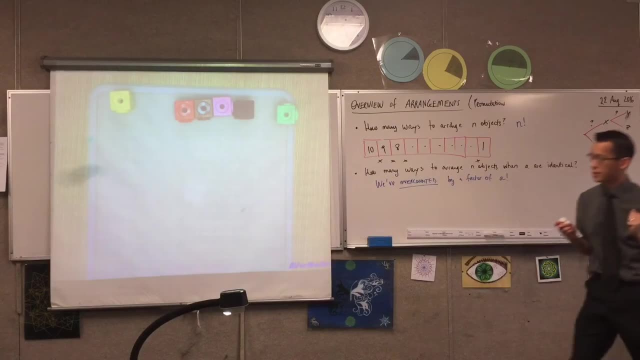 and still be in there and still look the same to me. okay, So they're still there. It's not like I have. it's not like I've asked this, right, It's not like I've asked this. This is about how many ways to arrange six objects, which is six factorial okay. 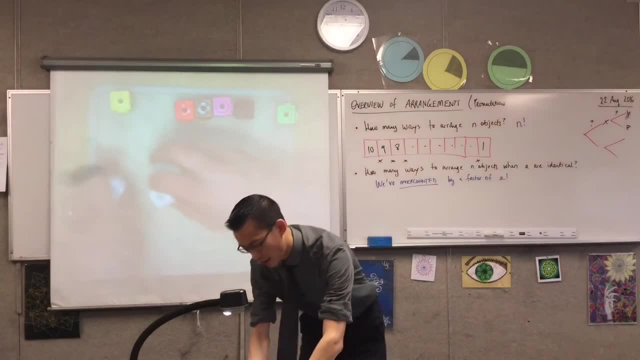 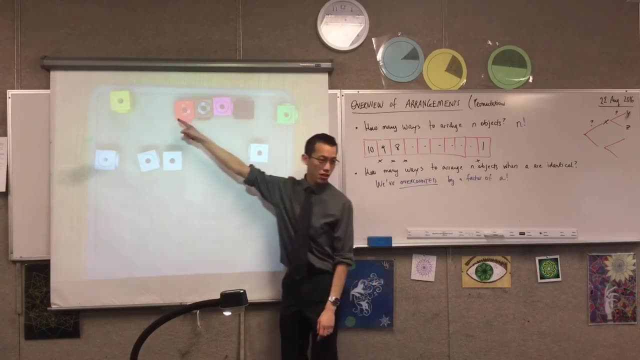 But I've got. I've got more ways than that. Like I've got, I'm still including these guys because, remember right, Including them in means I can arrange these guys not just in the order they're in now. 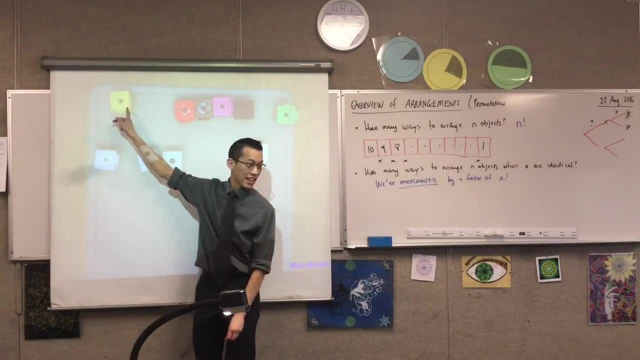 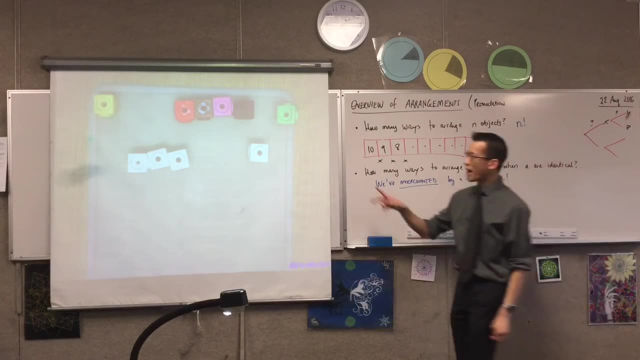 but I can put them in different spots, Like, for example, see how this guy's second at the moment I could make him first and that's that's new there. Good morning, okay. So whereas what you're thinking of like actually removing these guys all together. 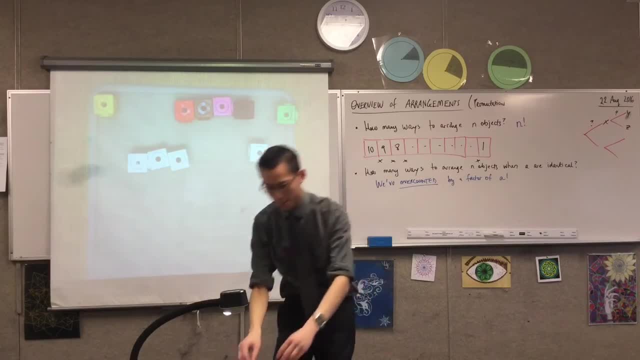 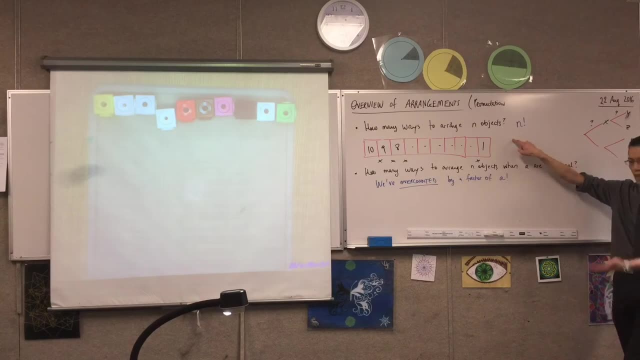 and just leaving with these. that's six factorial, but this is still including. I still have ten spots to fill. I'm still doing this. I just noticed that some of them, some of my lines of ten, look the same, and so I've overcounted them, okay. 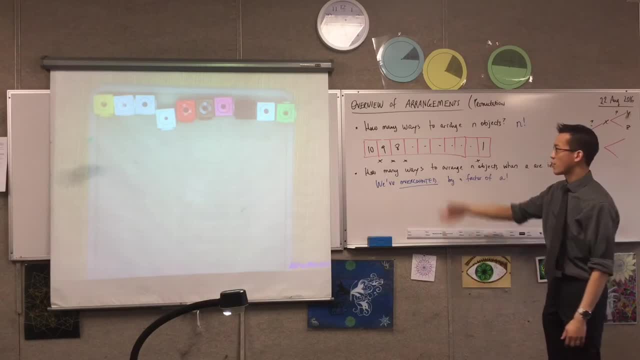 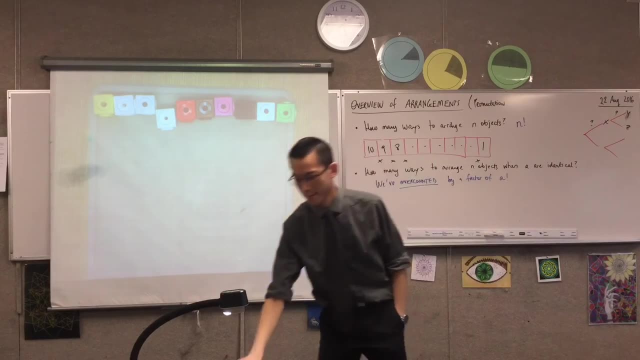 So it's not about arranging less objects, it's about arranging the same number but realising that some of those are the same. okay, How are you concentrating before I position over white inside the colourful ones, Like, for example, if I've got all four of them, which are the white ones? 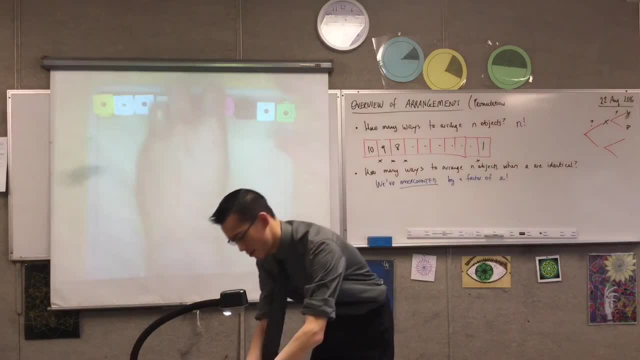 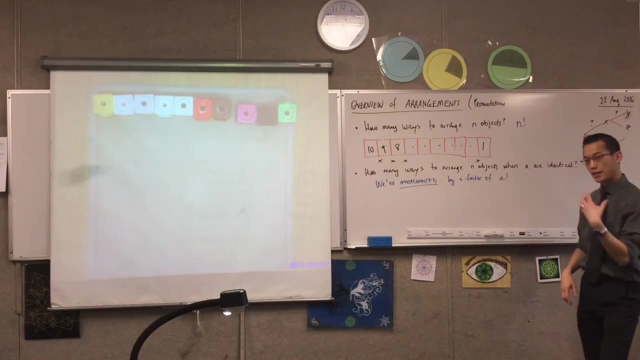 and I've got them right in the middle next to each other. where are we concentrating on that? Yeah, okay, so the answer is I don't need to compensate, because I've counted all the different ways I can put them, say: 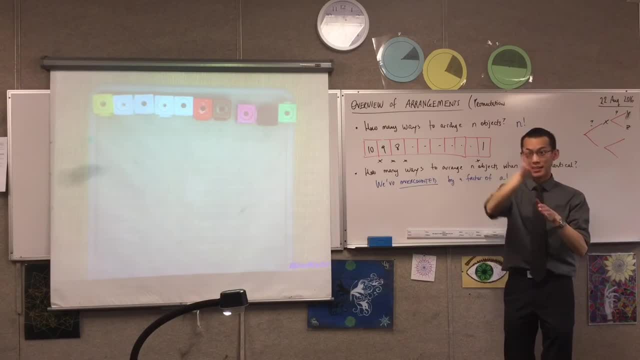 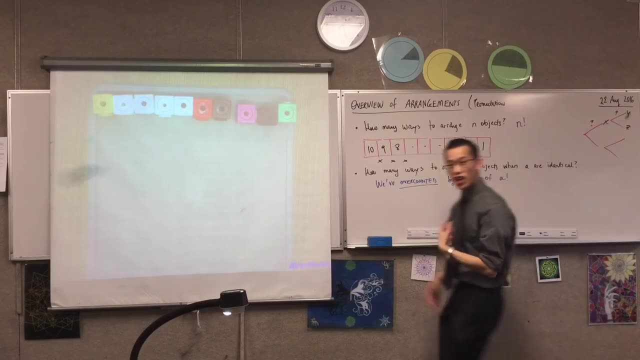 all together or separate or like interleaved between them here, right, When I just thought about where am I going to put these guys. it's ten factorial, It's just that like, so I've got, I've got this arrangement and I've also got this arrangement right. 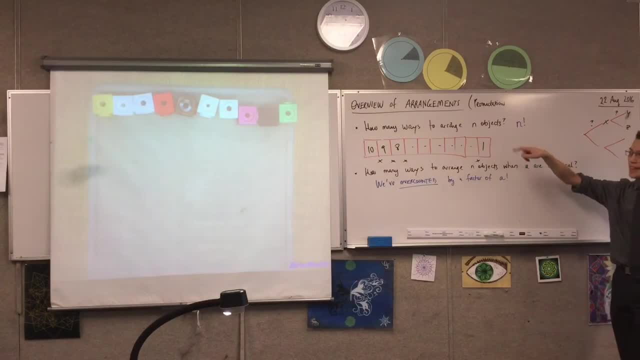 Those have been counted here right, But then these look identical to some of the other ways I could do this, like if I yeah that's right, if I gave these guys names right And then and started rearranging and I knew they were different but then took off all their labels. 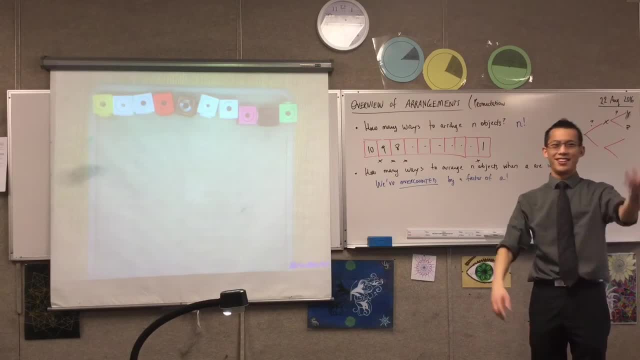 and was like: well, it's the classic sort of like twins experiment. right, It's like you know anyone would be like let's just have the same haircut for a little while and be able to swap back and forth. 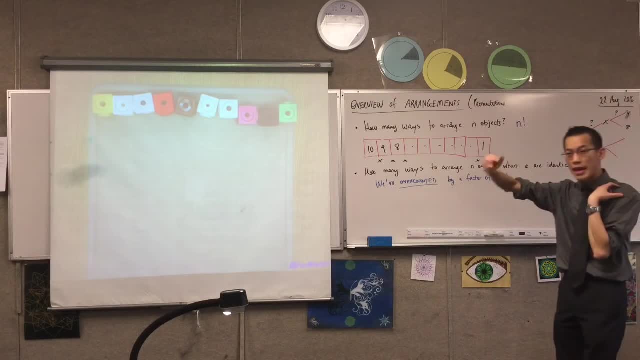 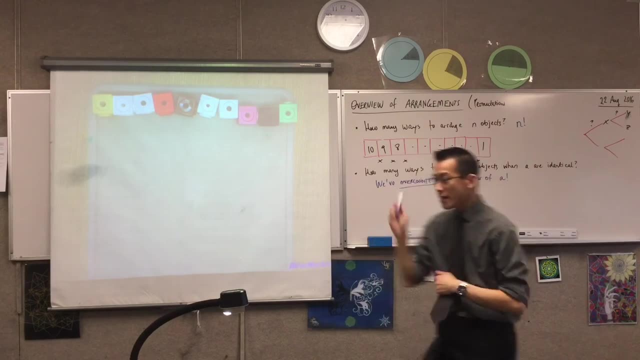 But well, we can't tell the difference, mostly, okay. So that's what I'm worrying about: The positions have been taken care of here and I'm worried about the over-counting here, okay, So. so therefore, because I've over-counted right, I start with my n factorial, which was ten factorial in this case. 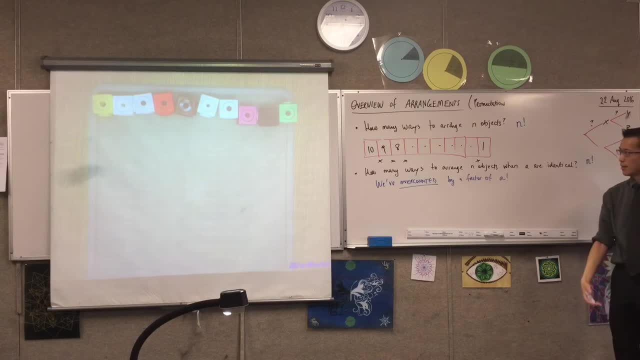 but because I've got too many, in the same way that you argued for me. hey, you better be multiplying here, not adding to compensate. I'm going to divide. That's the opposite of my multiplication operation, right? So that's n factorial on n factorial, right. 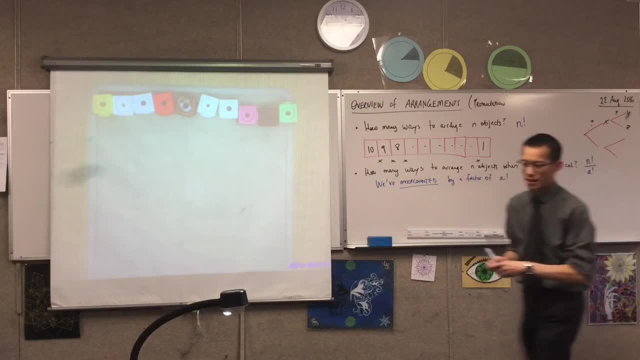 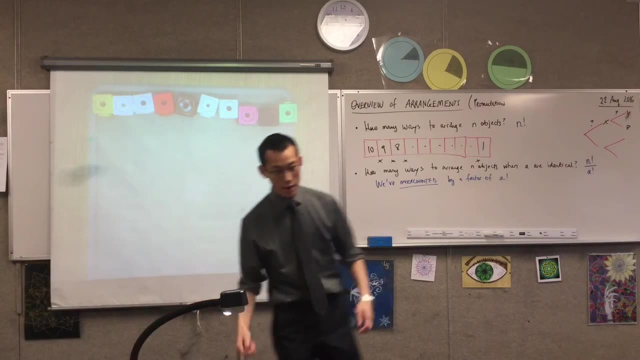 Now, the reason why I chose a is suppose, now, I didn't ask you to do this because this is a bit excessive Suppose. I then said, okay, it's not just, for example, four. I didn't ask you to do this because this is a bit excessive Suppose. I then said, okay, it's not just, for example, four. I didn't ask you to do this because this is a bit excessive. 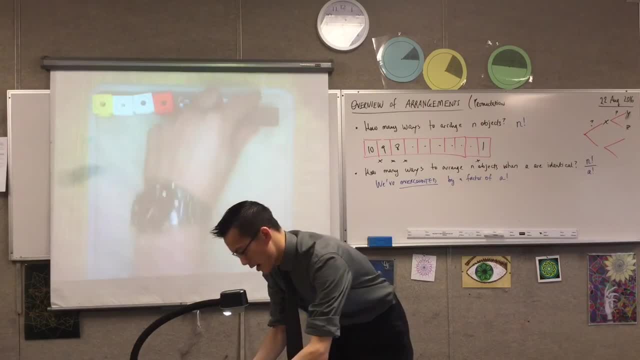 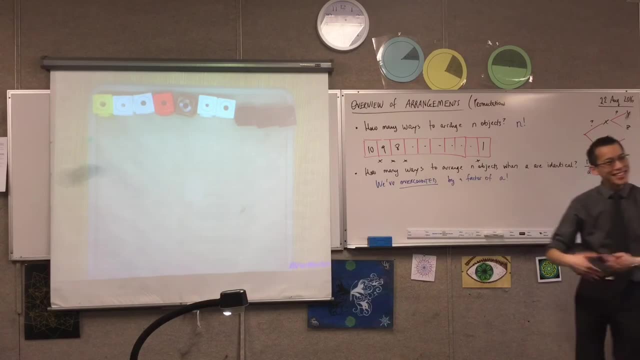 Now here's my n equal object. I might have four of those and three of these. okay, Now I can still rearrange those four white ones, right? But then, in addition to that, as well as that, I can rearrange these black ones, right. 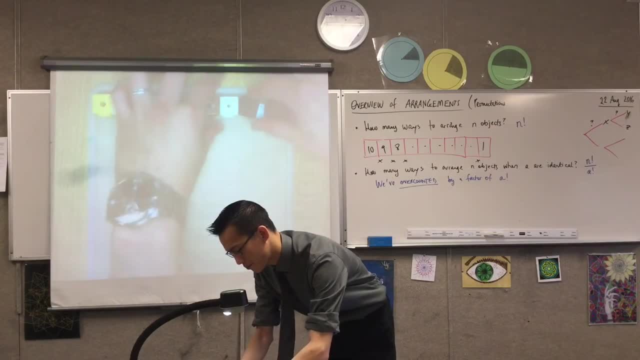 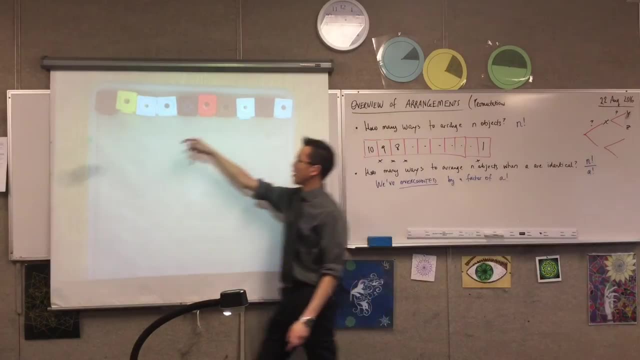 So actually I'll put them separate so you can see them a little clearer. So when I have a look at this, I could swap this one and this one, just go end to end, right, And it would still look like the same arrangement to me. 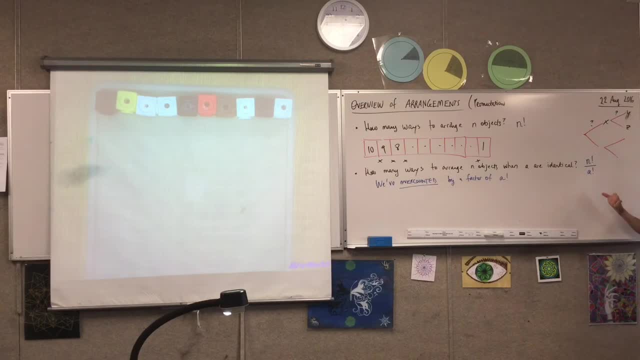 So, as well as doing the A factorial and having overcounted good morning by that factor, I could overcount by a factor of, say, B factorial. if that was like, that might be 3, and A factorial and B factorial and C factorial. however many identical elements I've got. 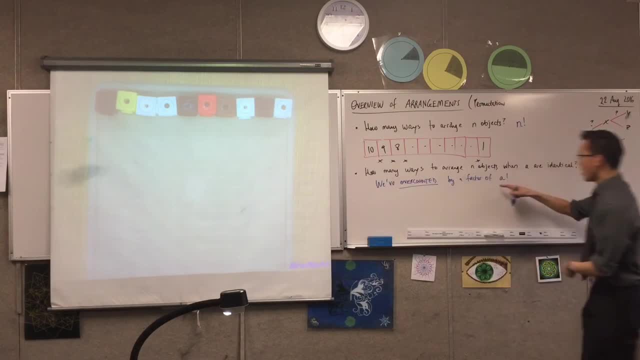 So maybe you want to make a note of that- Not only by a factor of A factorial or B factorial, C factorial, etc. according to how many kinds of identical elements I've got right. So would you just divide a factorial by those other ones? 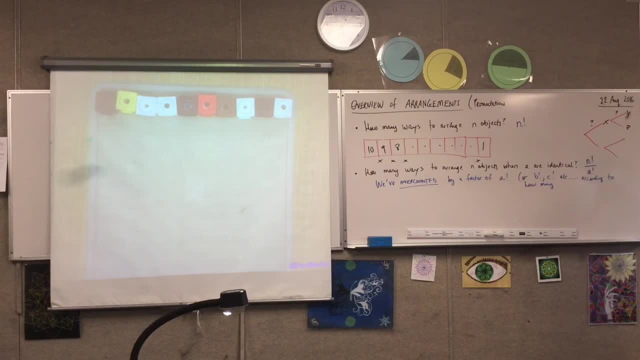 Yeah, exactly. So, for example, this one here would be 10 factorial on 4 factorial, 3 factorial right. Because again, think about this Now- I had before remember I pulled out these four and I said: